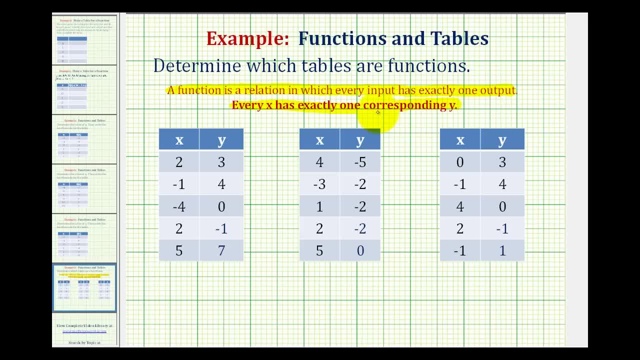 corresponding y value. If this is not true, the table would not be a function. So we want to analyze these tables and make sure every x value has exactly one corresponding y value. So if we take a look at this first table, notice that the input of 2 occurs twice. 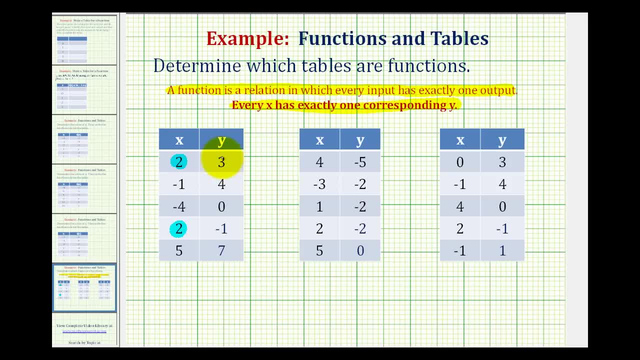 with two different outputs. Here we have an input of 2 with an output of 3, and here we have an input of 2 with an output of negative 1.. This does not satisfy the definition of a function, because the x value of 2 actually has two different outputs. 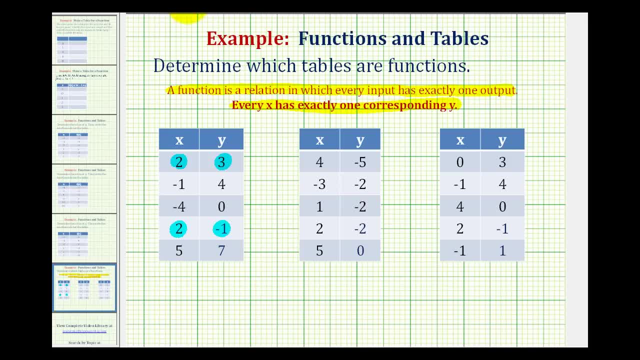 or two corresponding y values. Therefore, this would not be a function To help visualize this. it's often helpful to show the relationship between x and y using mapping, which means we put the set of inputs here or the domain here and the set of outputs. 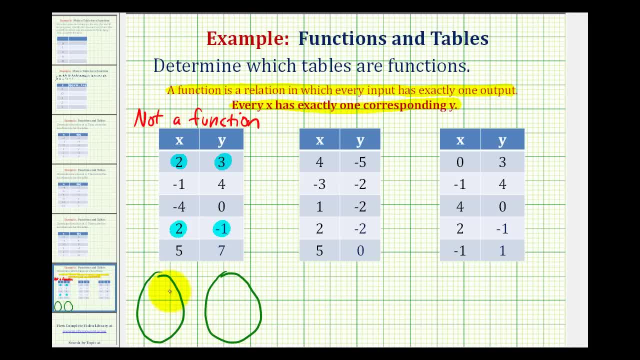 or the range here, and then draw arrows to show each input with the corresponding output. So notice our inputs would be 2, negative, 1, negative, 4 and 5.. We would not list 2 twice, So we have 2, negative, 1, negative, 4 and 5.. 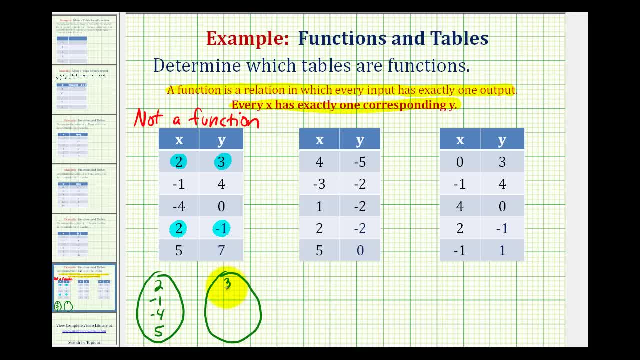 And the outputs are the y values. So we have 3,, 4,, 0,, negative 1 and 7.. So when the input is 2, here the output is 3.. So we show that relationship by drawing an arrow from 2 to 3.. 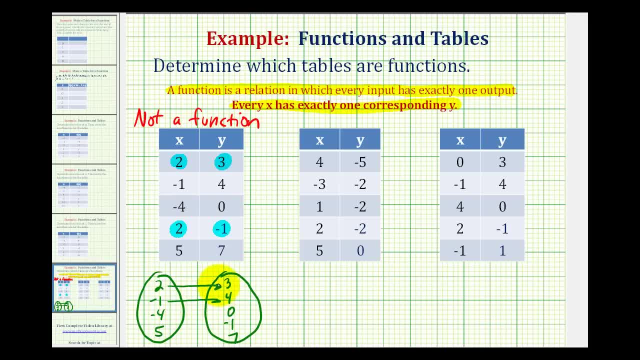 When the input is negative 1,, the output is 4. And the y value is negative 1.. So we would not list 2 twice. So we have 2, negative 1, negative 4 and 5. And we'll often say negative 1 maps to 4.. 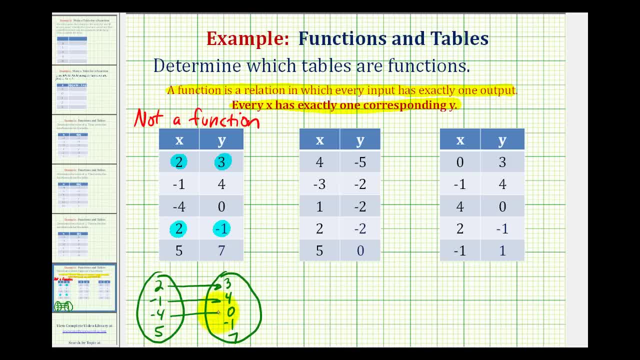 So we could say: negative 4 maps to 0.. But notice how 2 also maps to negative 1.. So we draw another arrow from 2 to negative 1 and then 5 maps to 7.. So notice that 2 has 2 outputs, 1 here and 1 here. 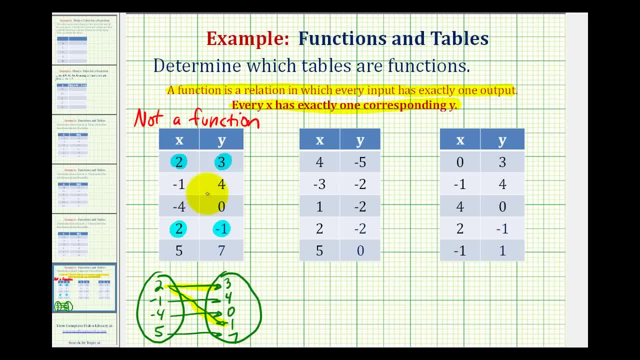 And this is the reason why this is not a function. Now let's take a look at the second table. Notice that none of the inputs here repeat themselves. Therefore, there's no way every x can have more than 1 corresponding y value. 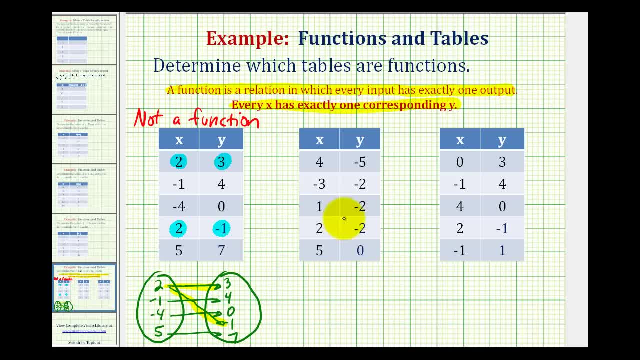 So this will be a function, but we'll also map it to illustrate it better. So again, we'll put the inputs or the elements or numbers in the domain here And then we'll put the elements or the numbers in the range here. 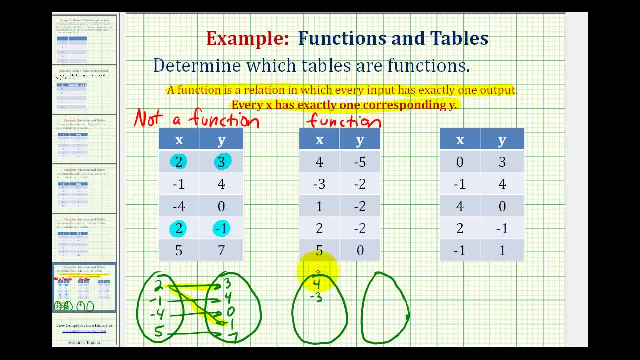 So the inputs would be 4, negative, 3,, 1,, 2,, 5.. And notice there is some repetition in the output. So there's only 3 outputs: negative 5, negative 2, and 0.. 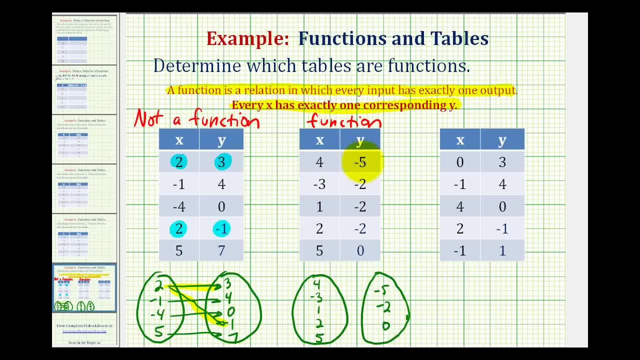 Now let's go ahead and show the mapping With an input of 4, the output is negative, 5.. So 4 maps to negative 5.. Negative 3 maps to negative 2.. 1 also maps to negative 2.. 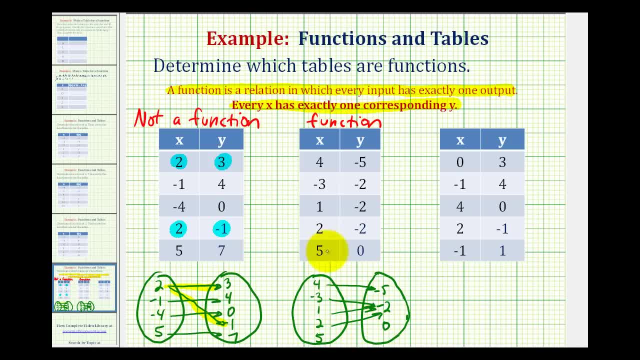 2 also maps to negative 2.. And 5 maps to 0.. Now this does look strange because we have 3 arrows all pointing to negative 2 in the range, But notice how every input or every value here does have exactly 1 output. 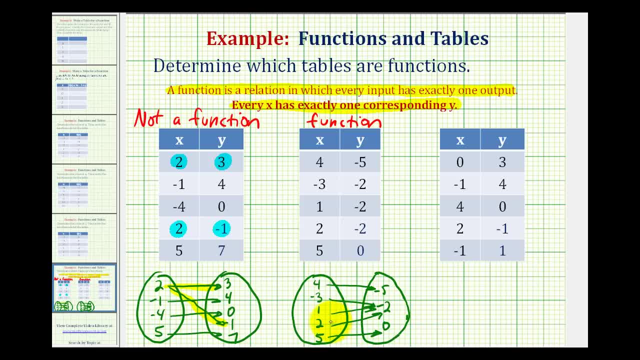 even though at times they do have the same output. So because every x has exactly 1 y, this is a function. Now let's take a look at one more example here. The first thing we should notice in this table is that the input of negative 1,. 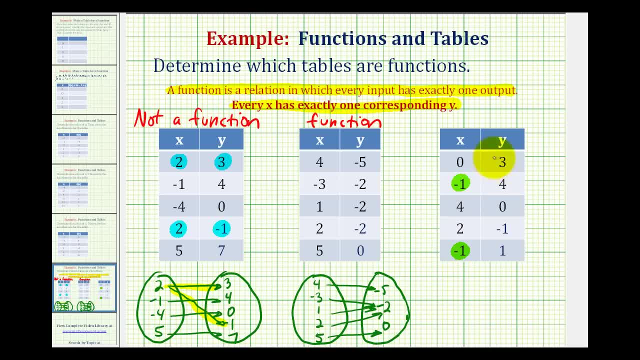 does occur twice. So negative 1 does have 2 outputs or corresponding y values. Therefore, again, this table is not a function And let's go ahead and map this as well. So the inputs are 0,, negative 1,, 4, and 2.. 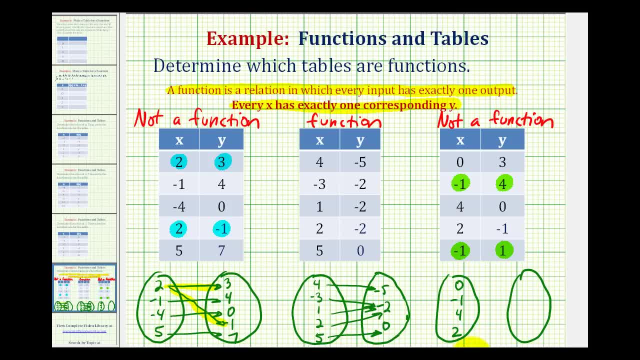 Again, we do not list negative 1 twice, Then the outputs will be 3,, 4,, 0, 1, 1.. zero, negative one one. So zero maps to three. negative one. maps to four. four maps to zero. two maps to negative one. 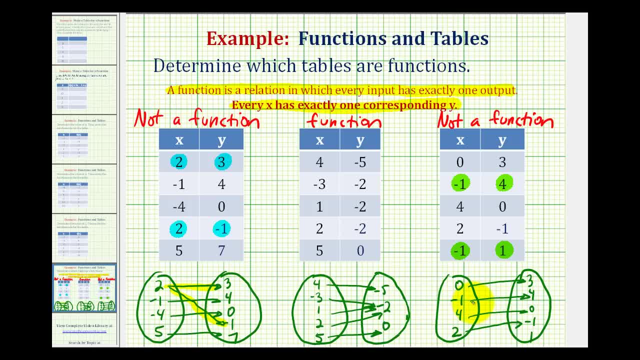 and then negative one maps to one. So from negative one we have another arrow going from negative one to positive one. So again, because this input of negative one has actually two outputs, this table does not represent a function. I hope you found these examples helpful.